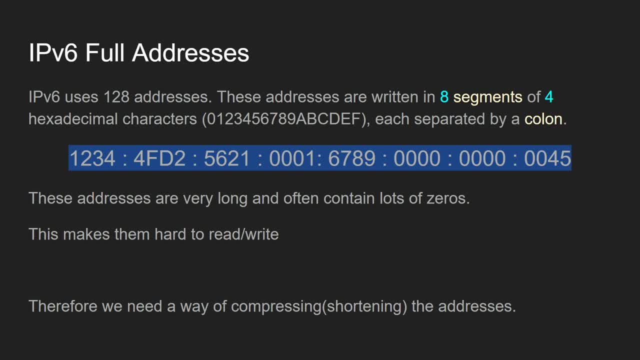 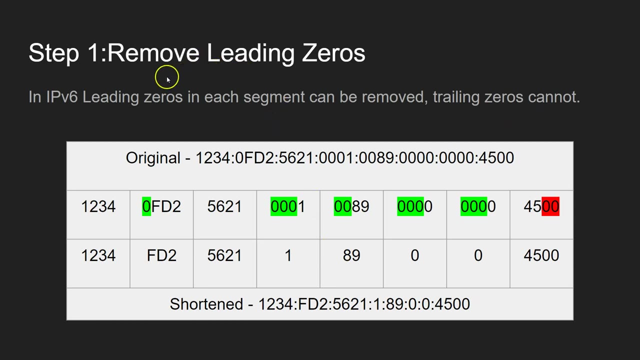 compress those addresses where possible so that it makes it easier for us humans to handle, and that's where the IPv6 compression comes in. So there's a number of different things that we can do, and the first thing that we can do is we can remove any leading zeros inside of a segment. So here we've got a. 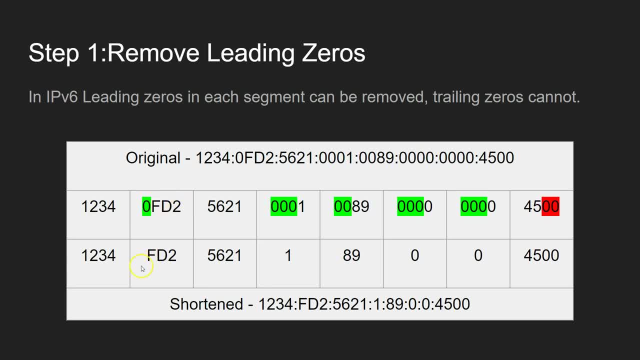 leading zero there in 0 FD2, so we can just use that as FD2.. In there we've got three leading zeros, so we can just replace that with a 1.. Two leading zeros, replace that with 8,, 9, etc, etc, and you could do that with all of the leading. 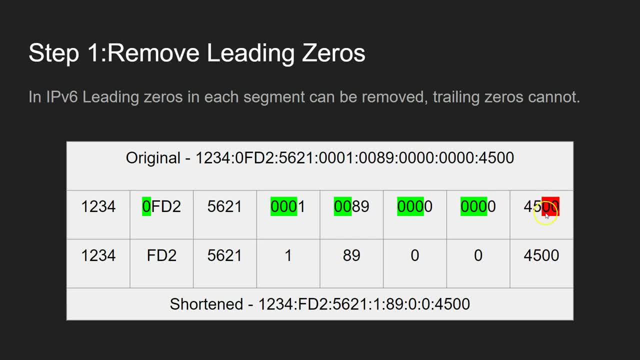 zeros, but you cannot do it with any trailing zeros here, And the reason being is that removing leading zeros doesn't change the value of the actual number. So 0 0 0, 0 is the same as 0, because it's just 0 and same here. 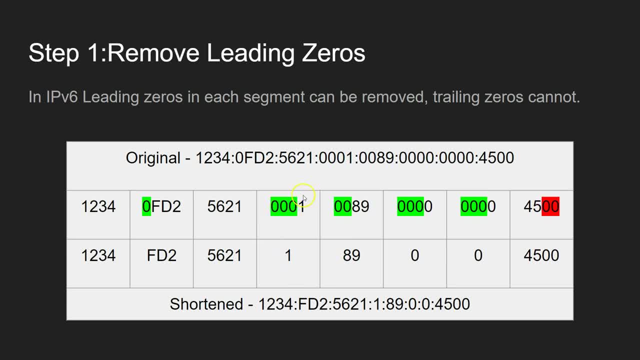 just like 0, 0, 0, 1 is the same as 1.. It works the same in hexadecimal as binary, as normal binary numbers. So we can't get rid of the trailing zeros because 4, 5, 0, 0 it's not the same as 4, 5.. But we could do it to most. 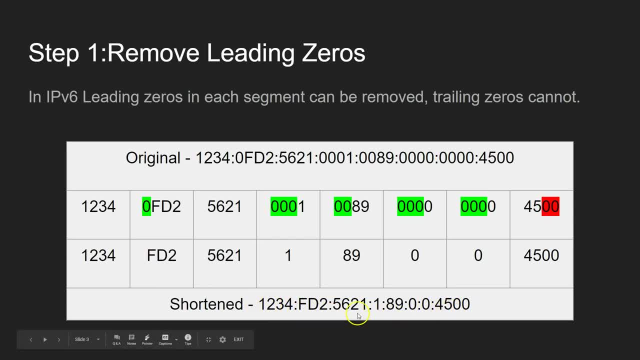 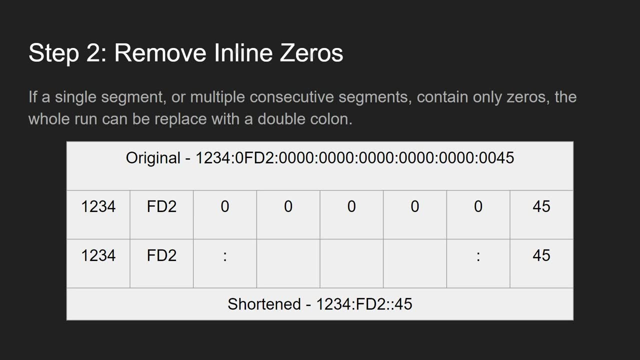 of it and, as you can see there, the shortened version of the IP address there at the bottom is quite a bit shorter than the original. But there's some more clever tricks that we can do as well, So let's have a look. So the next thing we can do is we can remove entire segments of inline. 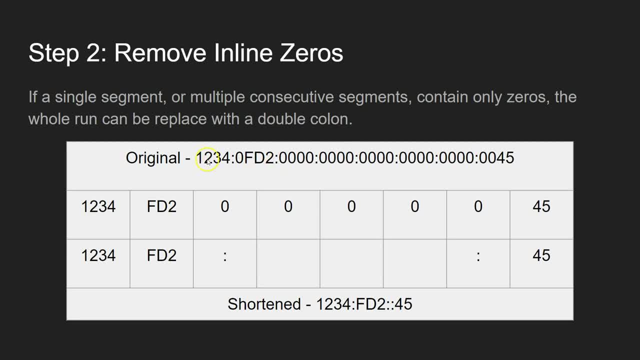 zeros. So if you look at this IP address here you can see is you've got 1, 2, 3, 4, 0, FD2.. And then you've got 1, 2, 3, 4, 5, whole segments where there's nothing really in. 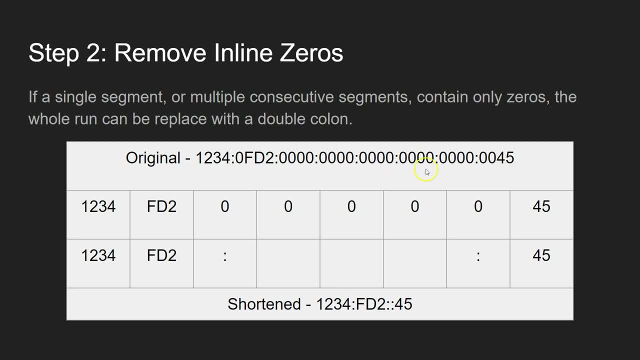 there of any interest. So what we can do is we can completely get rid of those segments, And the way it works is, first of all, we just shorten down the original here. So 0 FD2, that just goes down to FD2.. 0, 0, 4, 5 can be shortened down to 4, 5.. 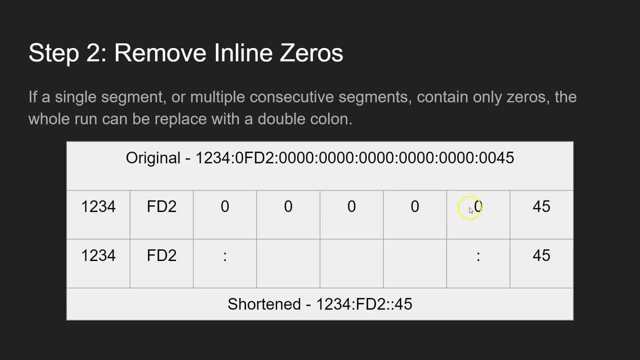 And this entire run here of zeros can just be replaced with a double colon: colon at the start here and a colon at the finish here. So the whole thing shortens down to 1, 2, 3, 4, FD2, double colon and then 4, 5. Which is much. 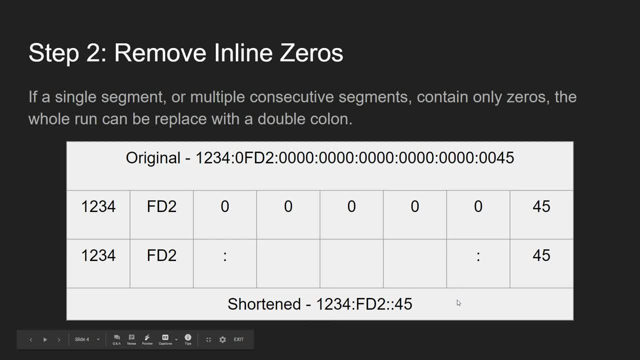 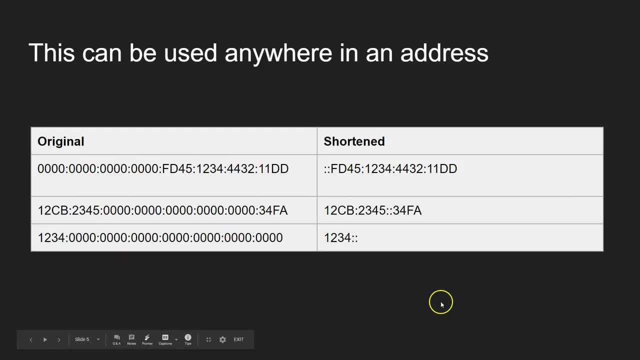 much easier to read, almost comparable to a IP version 4 address. So let's have a look. Let's do a few examples Now. a few examples here. this it's important to note, this- can be done anywhere within the address. so for instance, here: 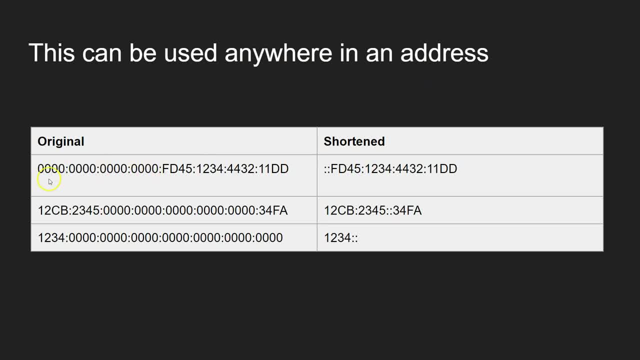 it can be done where there are empty zero segments here at the start of the address. so you just get rid of all the zeros and put a double colon at the start to indicate that the beginning is all zeros. we can do it here in the middle. so just like in the previous example. 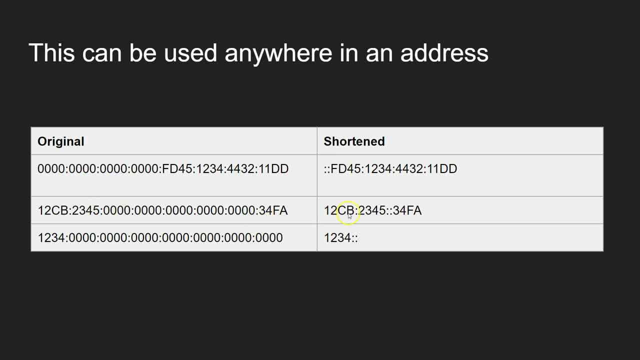 pop down the numbers that we need and then do your double colon right through and then have the last bit there, and it can also work at the end. so if there's nothing at the end here, if that's all zeros, then just put your star and a double colon there. 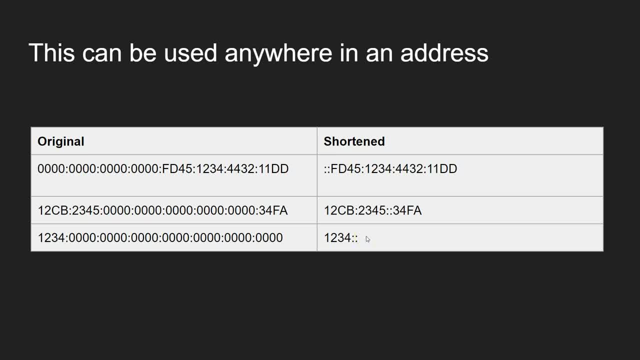 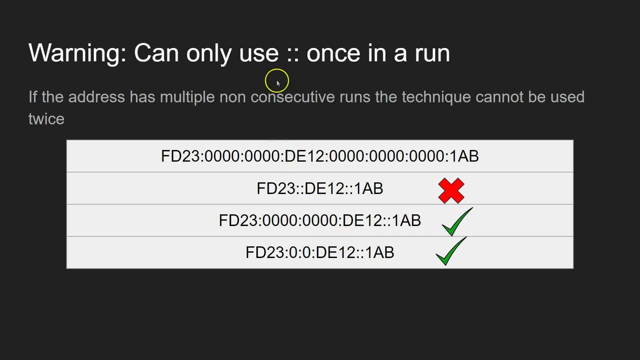 so it really does shorten these IP addresses down significantly. and there's a few points to note, though, and that is, you can only use a double colon once in a run, and so, if you look, here, we've got FD23, then we've got a run of. 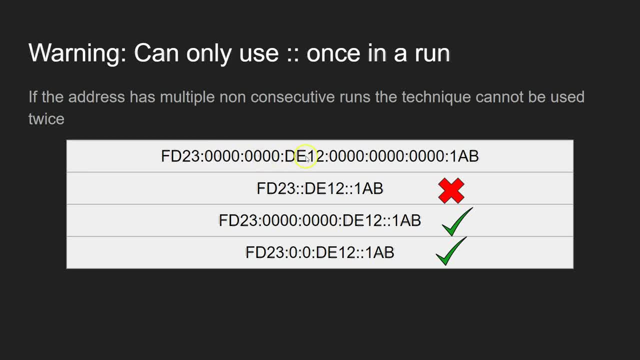 two segments of zeros, followed by a number, followed by a non-empty one, followed by a run of zeros. here you can't do two lots of colons, and the reason being is that when you come to decompress it, you have no idea where these zeros go. 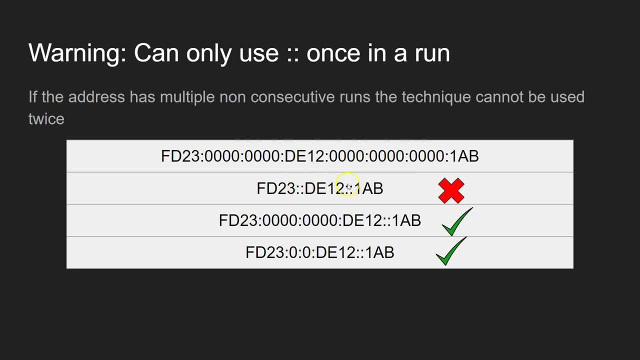 you know there's going to be some zeros here and you know there's going to be some zeros here, but is it one segment here and then four segments there? is it four segments here and one segment there? two and three, three and two, et cetera? you don't know. so we